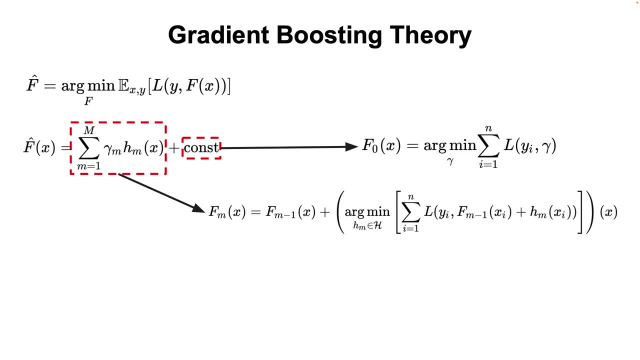 in order to improve our prediction and minimize the loss. Let's iterate again so you can better understand this statement. So we have our current approximation, fm-1, and we are trying to improve it and obtain fm To do that. we are thinking for a weak learner, hm, that when added to f, minimizes the loss. 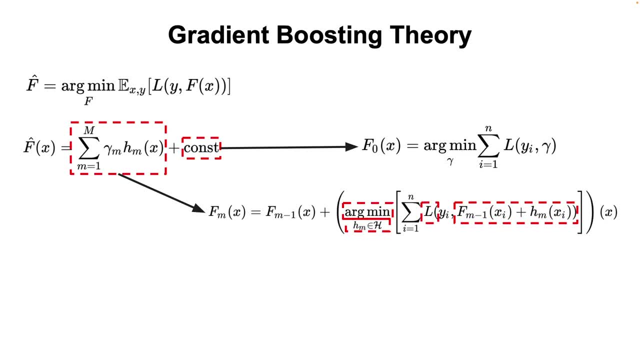 between our predictions. We can also compute the loss with a reduction of f, And so we have our new expression f, which is probably a little bit better, and we can use it to show that a weak learner is not a good student. 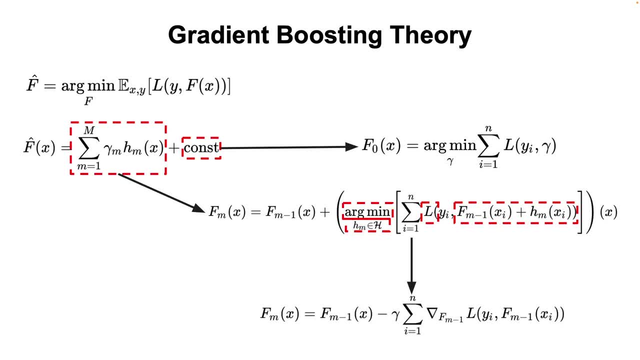 So we can just add some expressions and labels. Unfortunately, it is not computationally feasible to find the optimal weak learners in this equation, and the best we can do is to take a step in the steeper descent of this optimization problem. Henceforth the name of the algorithm: Gradient Boosting. 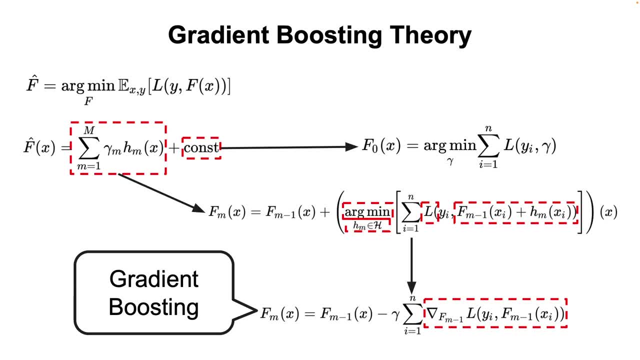 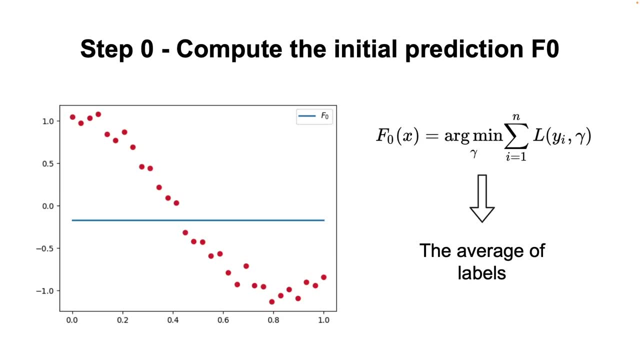 Ok, so that was the theory behind Gradient Boosting. Now let's look at the implementation that is used in most of the cases for this algorithm. As I said, the first step is to compute F0 and for regression, when the mean square loss is employed. 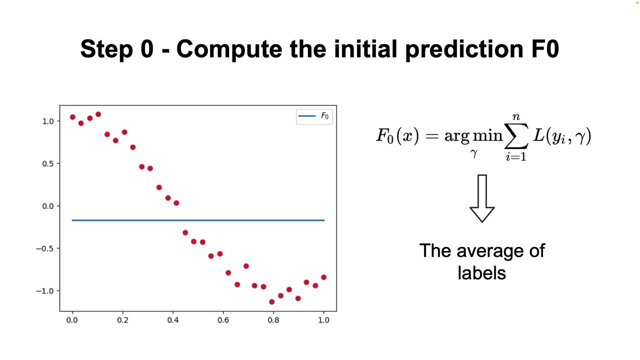 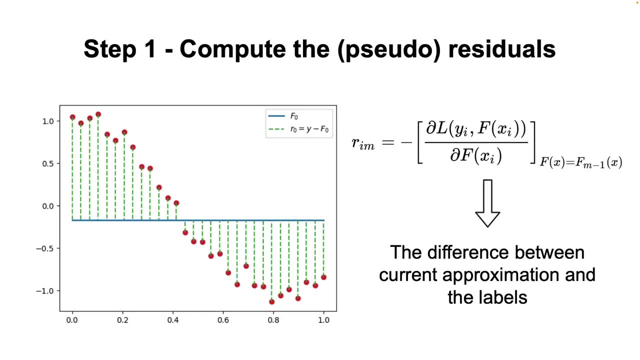 it is nothing else than the average of the labels. I've added some materials in the description that explain how this is derived for those of you that want to see more. The next step is to compute the gradient, or, as they are often called, in gradient boosting, the pseudo-regiduals For our study case. 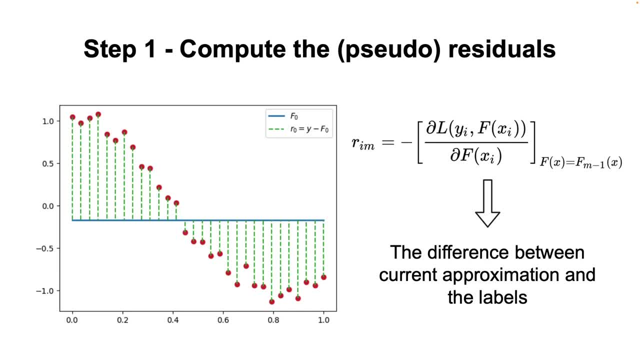 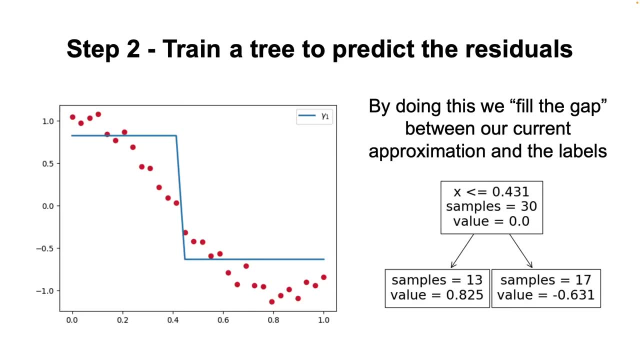 this is simply the difference between our current predictions and the labels. Again, if you want to see why this is true, check out the links in the description. Then we train a weak learner, our shallow tree, to predict the residuals. By doing this, we try to fill the gap between our current 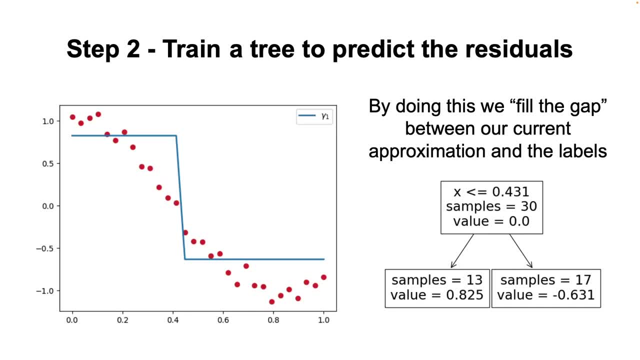 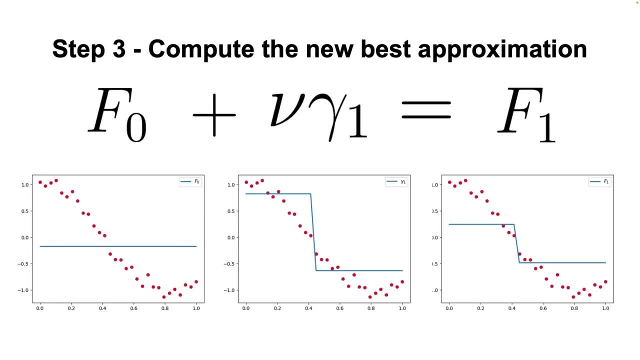 approximation F0 and the target labels, The predictions of the regression tree are denoted in general as gamma. Finally, we update our approximation F0 by adding the predictions of the newly trained weak learner. that is multiplied by a learning rate denoted as the greg letter, mu in this case, and thus obtaining the next approximation F1.. 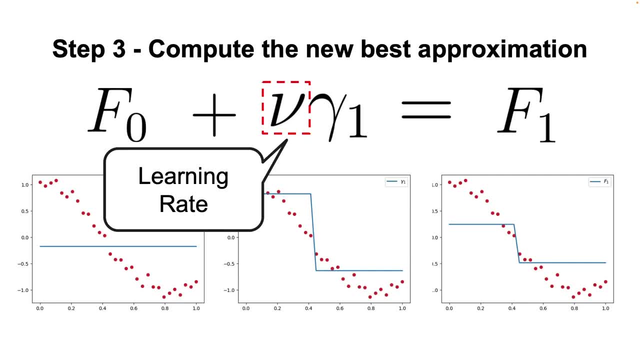 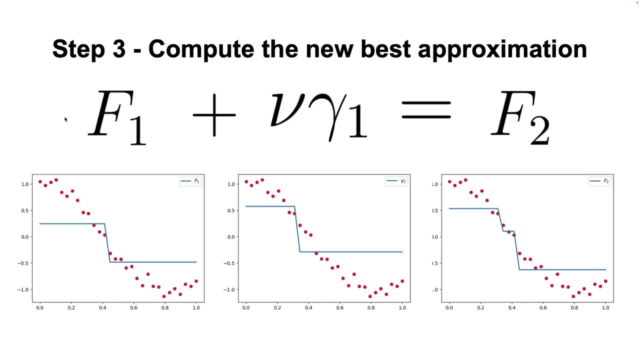 Now all we have to do is add more weak learners by using the last three steps. Let's try to follow these steps one more time just to see how the prediction changes. So we compute the residuals, then we train a new tree to predict the residuals, and then we add the.